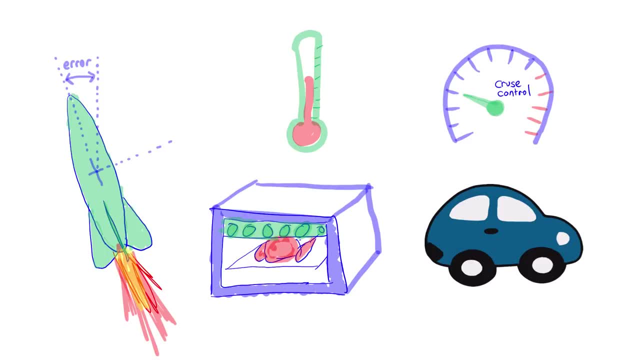 So control theory is something fundamental to most things, but it isn't always on the surface evident. Rockets are controlling for their pitch and yaw and other variables for stability, Ovens control for their temperature, And cars control for all kinds of things, but one of the obvious examples is cruise control, which controls for speed. 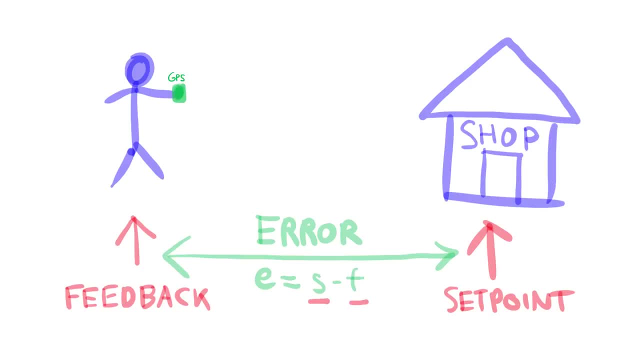 Even you, in your day-to-day activities, are a basic controller, or at least a whole ton of them. When you walk to the shop, let's say this is a guy here, Bob, walking into the shop with his GPS. he gets his coordinate from his geocaching GPS. It just gives you a. 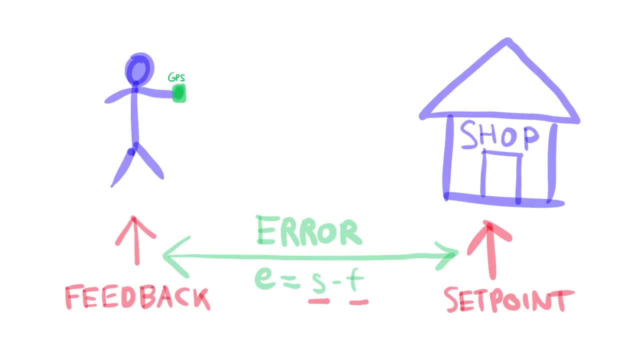 coordinate and he knows the coordinate of the shop and he can subtract the two, get the distance, and that distance to the shop is the error, which is basically the fundamental concept of control theory. Control theory is controlling and minimizing error. So there's a few things about error. Error is the set point, which is where you want to be, minus the 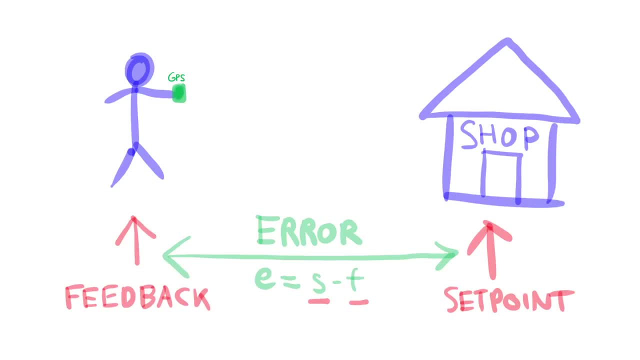 set point, which is where you want to be, minus the set point, which is where you want to be, minus the feedback, which is where you are. and this is an example with the position, but it doesn't have to be the case. It could be with speed, or it could be with acceleration or magnetic field strength, or 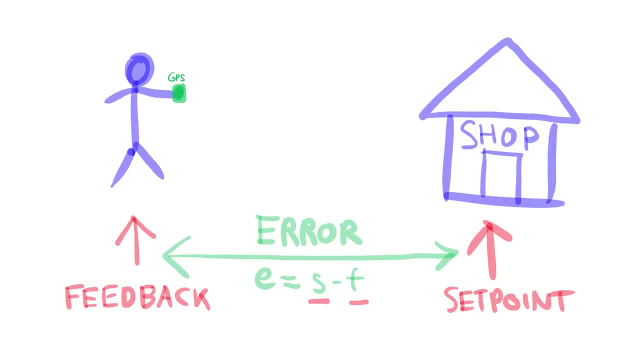 energy power. All kinds of variables can be controlled using the minimization of error or control theory. An error of zero would often be the position called the steady state position, and it is usually the goal. In cases where it's not the goal, I'm sure they'd be very happy with zero. 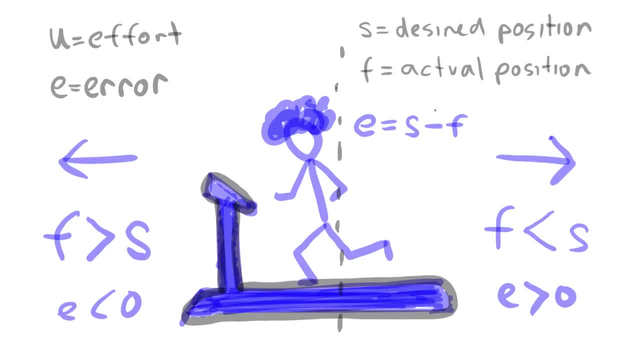 error anyway. After getting back from the shop, Bob realized that he'd eaten far too much chocolate, felt guilty and bought a treadmill. So on the treadmill he realized this is another element of control theory. He's controlling the speed of his feet, but what is he actually controlling? What? 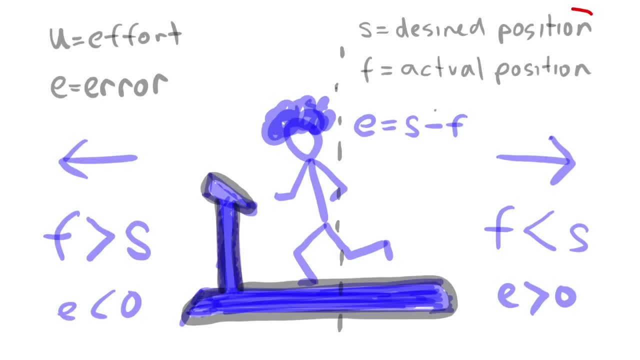 is he looking to do? Well, he's not actually controlling his speed, he's controlling his position. He wants to be in the center of the treadmill and if he starts drifting back, he knows he's not going fast enough. and if he starts drifting forward, he knows, he knows he's going. 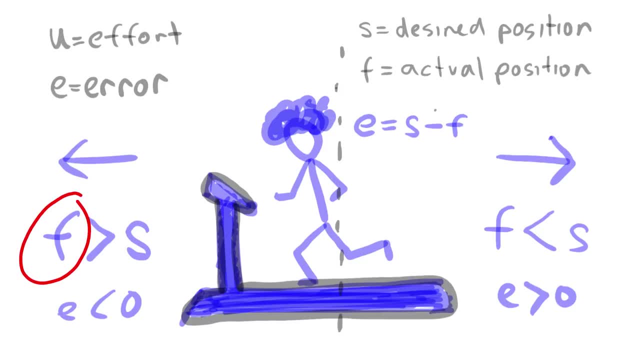 forward. So he's controlling the speed of his feet. So he's controlling the speed of his feet too fast. so that is, if his actual position is greater than his desired position, then he is, he's got an error less than zero if his actual position is less than his desired position. 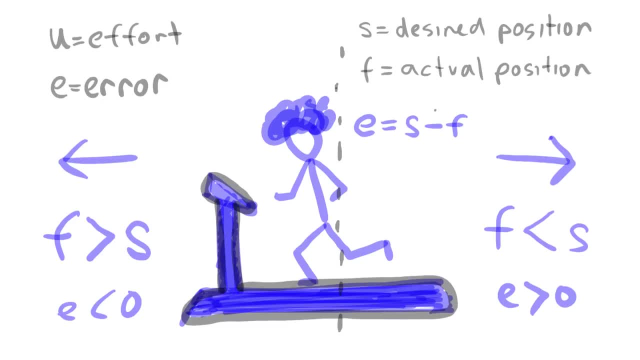 then his error is greater than zero and he should speed up. so what do we do with this error? well, we use this error to control effort, and effort is basically how much effort bob's putting on the treadmill. if he's not putting on in enough effort, he'll fly off the back and hit his head. 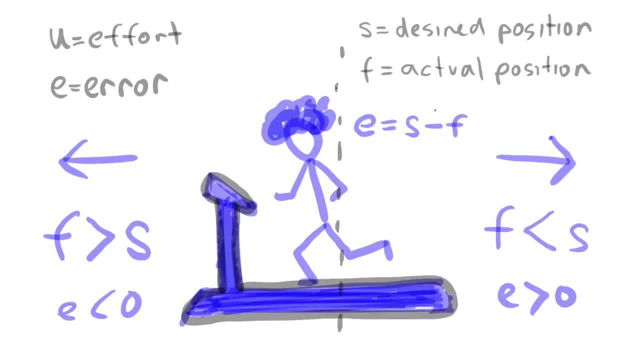 if he puts too much effort in, he runs into this stand thing here at the front, which so control theory is evident in basically all elements of things you do, from running to walking, to your body heat regulation, and while it may not be the a pid controller or any like formally represented. 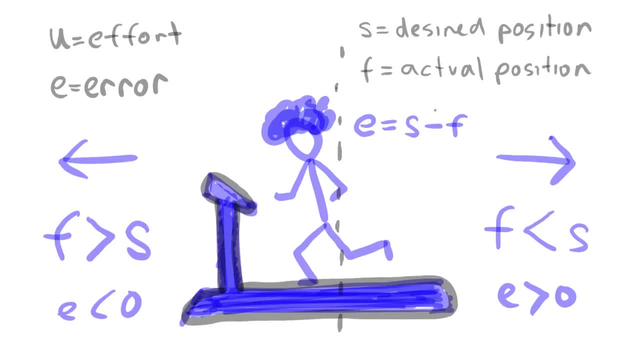 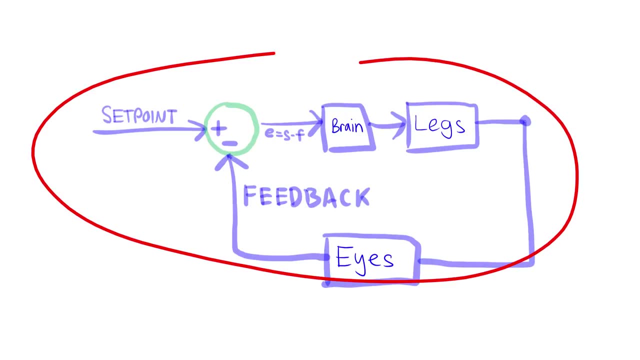 mathematical controller. it is explainable through basic control theory concepts. most control theory textbooks and lectures have diagrams- this throughout the entire book. This is a basic diagram which represents the two previous examples, where the set point is the position Bob should be and the feedback is the position Bob is. He gets that feedback from his eyes and he uses. 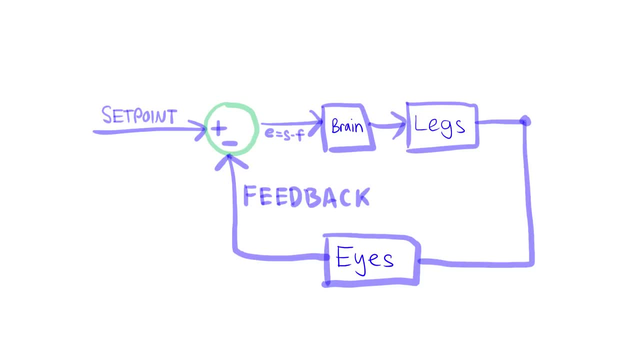 his legs to move him to different positions and his brain controls his legs and he looks at the error to make decisions with his brain. So if we go through that like this, you see why it's called a control loop- because it's a loop. It just goes round and round and round. and for control loops in digital 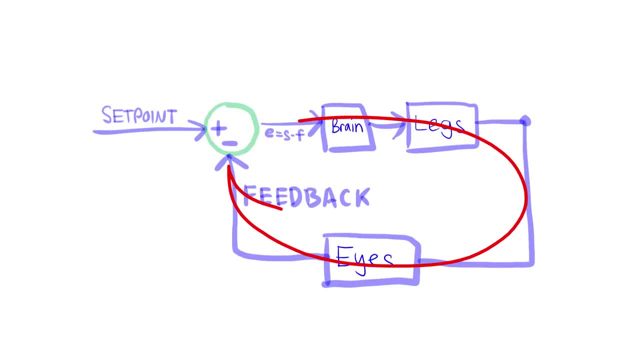 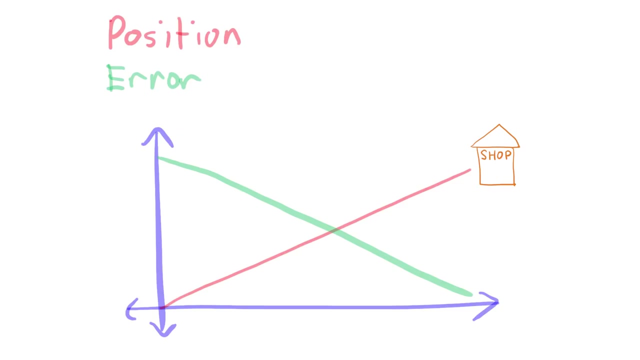 systems. it's usually a periodic loop. It goes round once every second, 10 milliseconds, something like that- which then makes very fast and sensible, hopefully, adjustments to the system so that the system is controlled. When Bob was walking to the shop, he's his position was going up the whole time, but his error was going down. 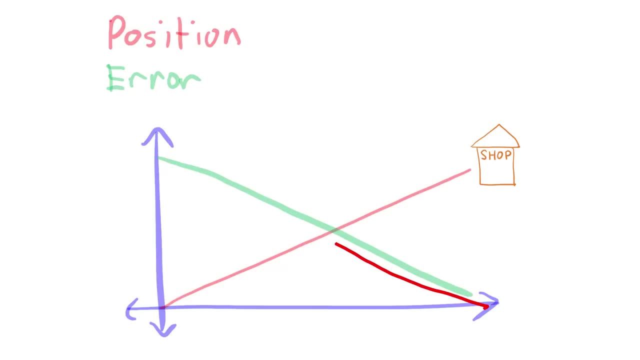 and that is what we want to do. we want to minimize error. So, up the top here, his position is equal to the initial error and if you look over here, and his error is actually the distance to the shop initially. so in this case the error units are in the same units as the position, which is, which is much simpler. 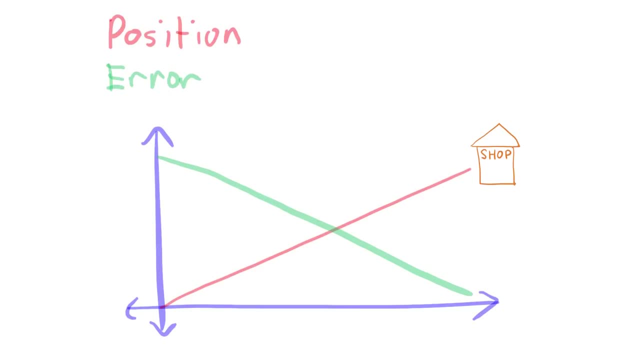 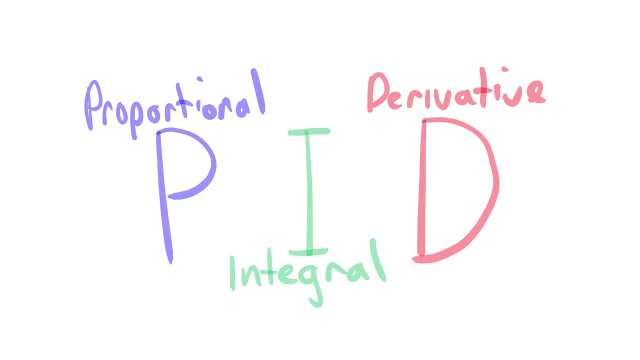 than it could be, Because sometimes you have to convert the units so that they equal each other and they're comparable. So one of the most common industry controllers is the PID controller, that's the proportional integral derivative controller. and these things are found everywhere, from motherboard fan controllers to heaters to balancing. 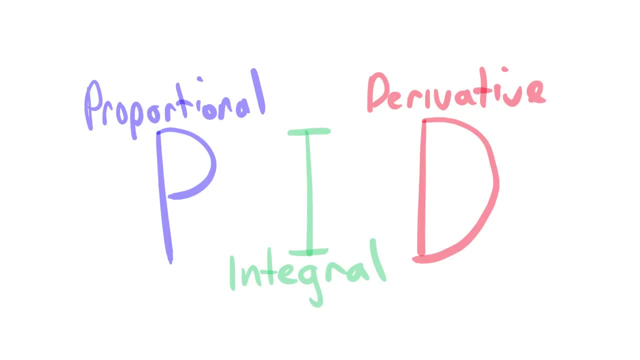 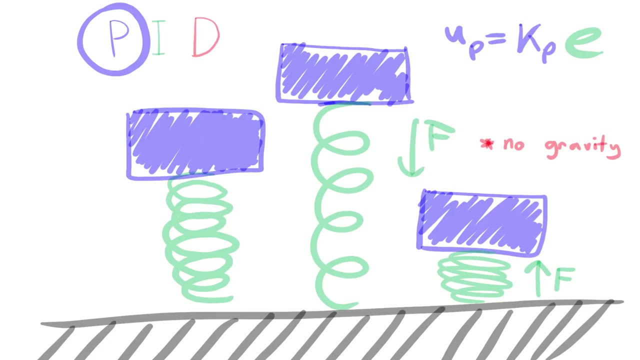 Segway things there and they're in all kinds of things and they're quite a primitive controller, but they're really easy to tune and pretty fast to get up and running. so we're going to talk about that, Okay, so a PID controller can actually be separated into three different. 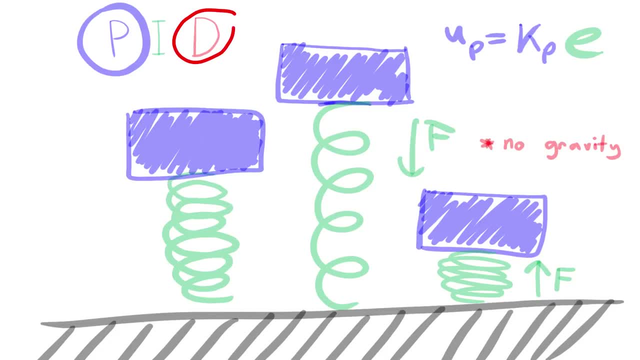 controllers: a proportional controller, an integral controller and a derivative controller. We're going to talk about a proportional controllers behavior. A proportional controller is actually analogous to a mechanical spring where the default position is when the spring isn't stretched or compressed and that default position would be the controllers set point If the controller 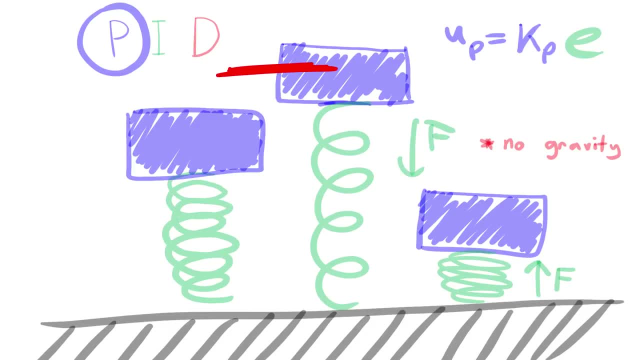 the spring was stretched, then the distance between the set point and the default point is the error. This is the error. When the error is negative, the force is negative. The controller outputs a force. in this case, When the error is positive, then the force is positive, trying to move it back to its set point. Now you'll 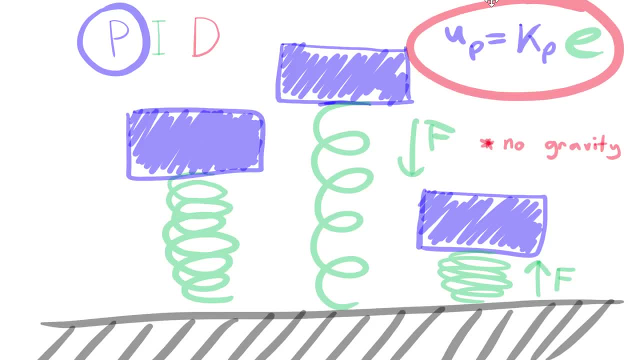 notice that there's an equation up this top corner here, and this equation should be quite familiar to many of you. It's the exact same form as Hooke's law, where Hooke's law is: f equals K, Delta X and Delta X in. this is really the difference of positions. but error is a. 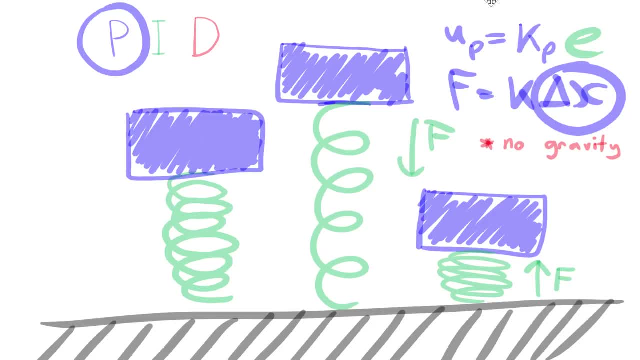 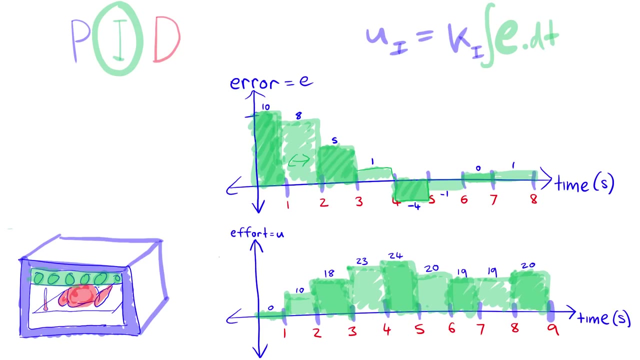 more general way of expressing differences of position. It's just the difference of an arbitrary unit, which isn't necessarily distance. So a proportional controller is basically an ideal spring. An integral controller can be used in lots of things and it's especially useful when you need to have 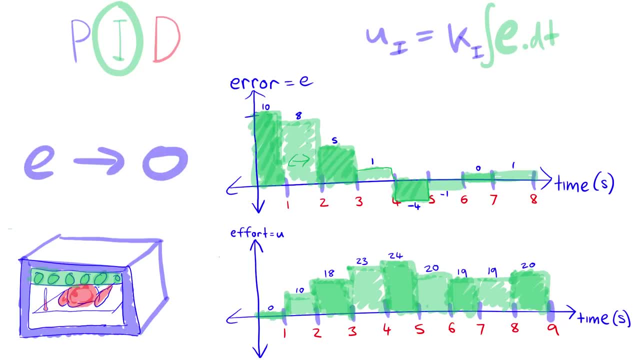 error eventually go to zero and these things, like they're in examples, like precision ovens and anything that balances anything, all kinds of things- require zero error because if there is any error, it ends up not performing to spec or ending up halfway across a continent if it was a plane or just it. 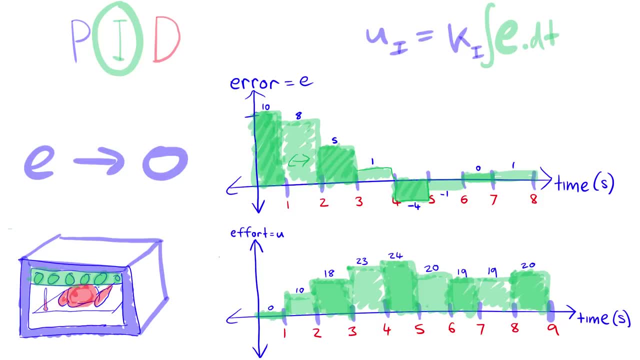 just ends up missing its target. so integral controllers are one of the more useful controllers for in scenarios where you need zero error. now we're going to talk about an oven controller. ovens aren't usually controlled with integral controllers. they they probably should be controlled with a thing called. 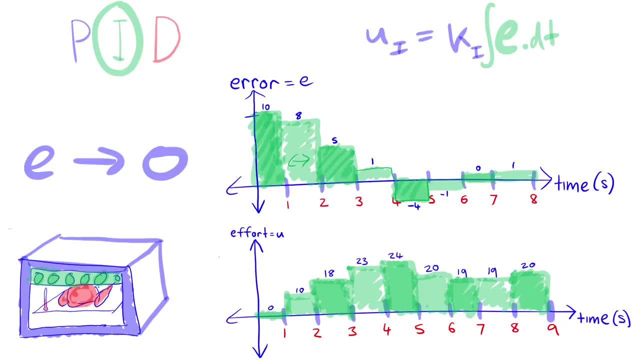 a bang-bang controller, because that is the scenario where bang-bang controllers are basically optimal. but but for this scenario, because it's simple, we're going to use an interval only controller- bit weird, but whatever anyway. so in this example we're trying to heat up. 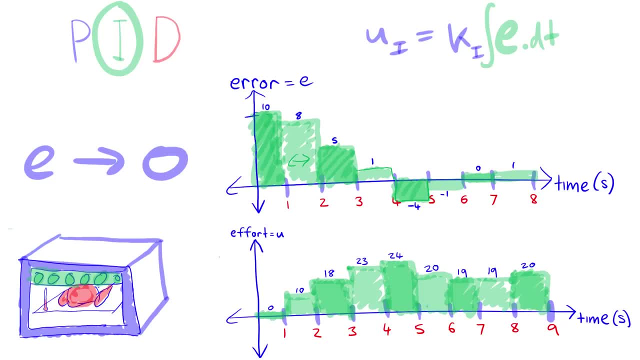 this oven and we're going to do it manually because it's not a very smart up and we just have this knob which you can turn. but we put a thermometer in the oven and we want to make sure that we're cooking our chicken at no, apparently I'm. 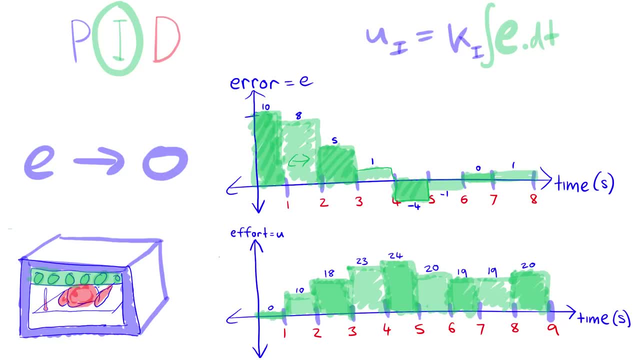 cooking it at 10 degrees, because that's what my plot says. we're cooking our chicken at 10 degrees, alright, anyway. so initially, the ovens temperature is zero because someone put it in the fridge and that would mean that the error is 10, the setpoint minus 0, the actual point. so that's here now, if you, 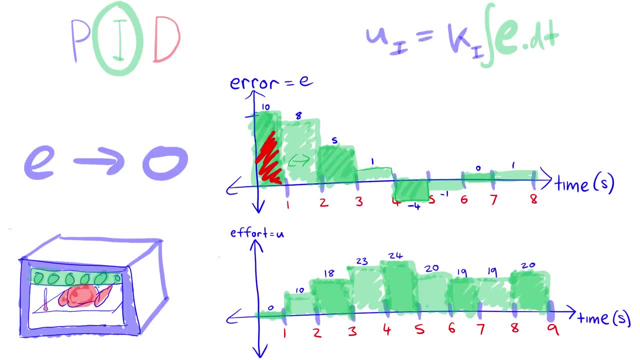 get the area of this error here, then that is equivalent to the integral up to time one, so our effort would be K times the that integral we just had before, and In this case the integral to the result is just 10, and for simplicity we're just going. 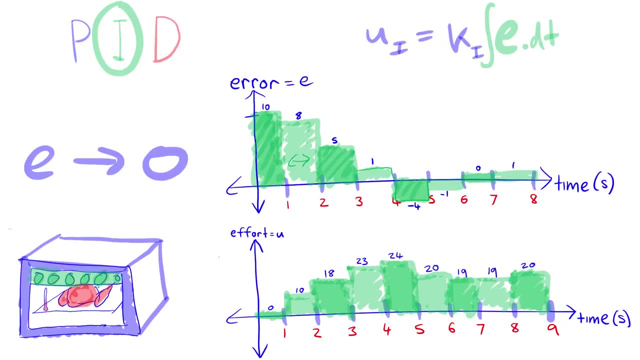 to have the constant out the front as 1,, but this can be anything. So initially our control effort u is 0, because we haven't actually started the controller, but after time 1, we're able to calculate our new control effort, which will be 10.. 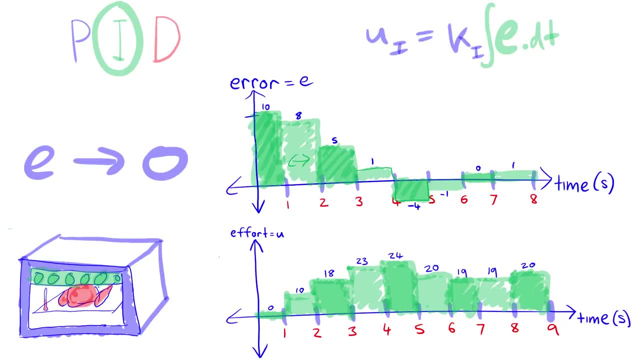 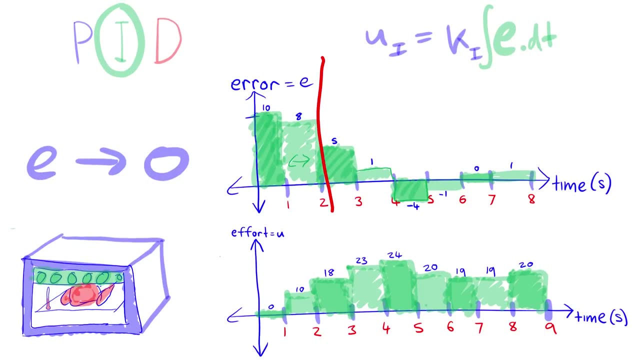 We then move forward the system by one more second and the oven has heated up a little bit because we've put a little bit of energy into the heating elements. Okay, so, after the first sample, we're up to this sample 2, we're taking a reading at the. 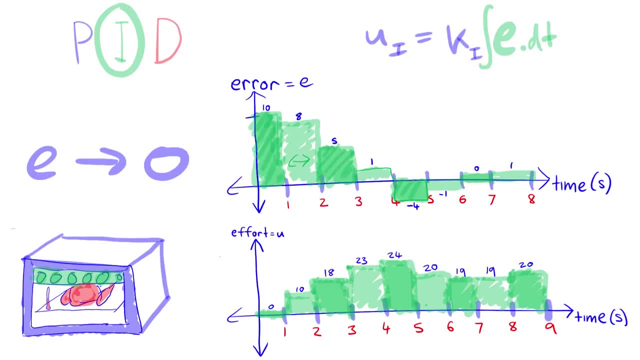 second. second: We now we've realised that the oven has gone up 2 degrees and that would lower our error by 2. So it was initially 10 degrees, and 10 minus 2 is 8.. Now integrals add up areas. that's how they work. 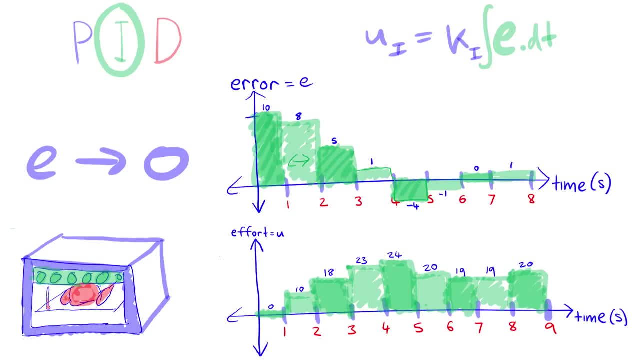 And so the The result of the integral In this case would be 10 plus the area here, which is 8.. So our next control effort for the next period between 2 and 3 will be 18.. And if you follow this through for a little while, the oven heats up more because we're 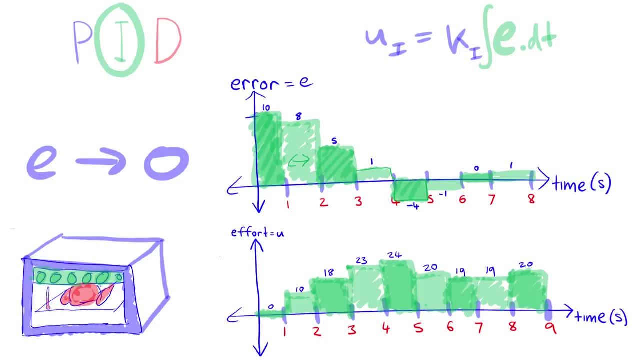 putting more effort in, we get 5, and we add the 5 to the thing and that results in a control effort of 23.. 23 is the area here plus the area here plus the area here, And the oven has heated up even more at this point. 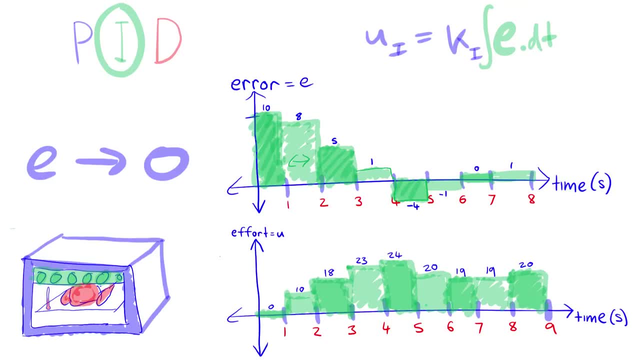 And the integral component is actually getting quite large And notice there's nothing driving the integral component smaller. that's very important And it's one of the biggest pitfalls of integral controllers, as we'll see in a moment. So the oven's temperature is now 9 degrees. 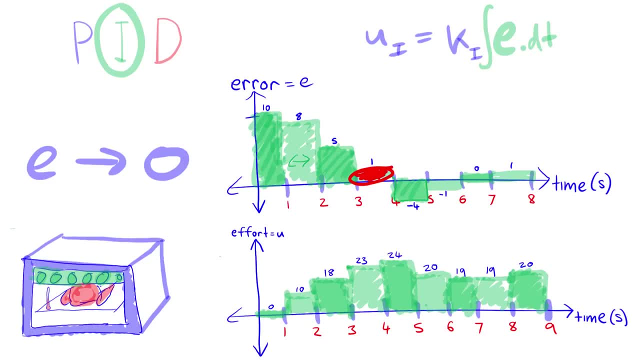 We have one more degree to go, so the error is 1, and we just add that to the result, So that's 24, the effort, And now we have all that accumulated area here And we're still providing an error of 3 degrees. 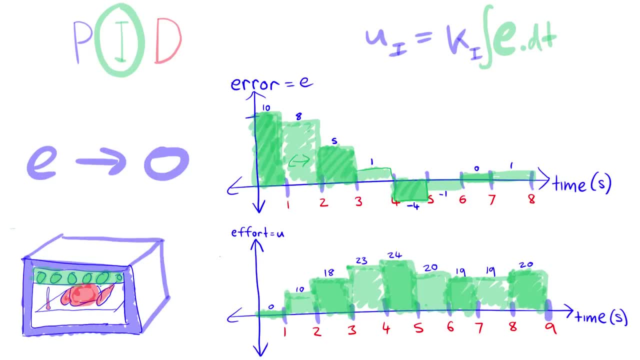 And we're still putting in the integral- probably heating up the oven, because even if you dial it up to 11, then it takes ages to heat up. There is thermal mass of the oven that takes a lot of time to heat up and that. 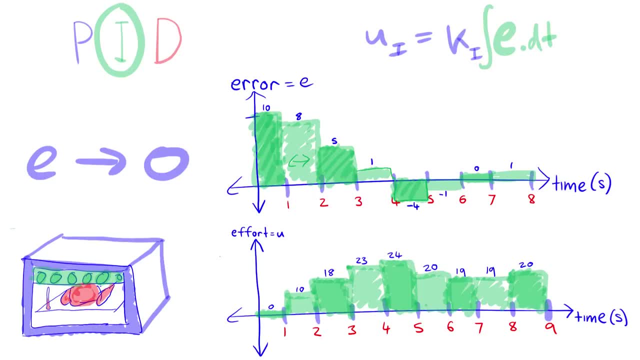 means there's a delay. The integral component has a very high value. now We're up to 24, and that means we're going to overshoot our set point. So in the next sample we unfortunately go to negative. we end up having an error of negative 4, because we've overshoot our 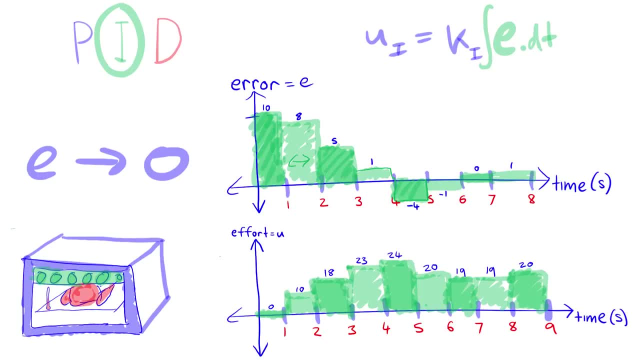 temperature. We're at 14 degrees, and 10 minus 14 is negative 4.. And if you add these areas to the negative 4 area here, then we end up putting an effort of 20.. The slight reduction in effort- because this oven has basically no thermal mass- apparently results in the 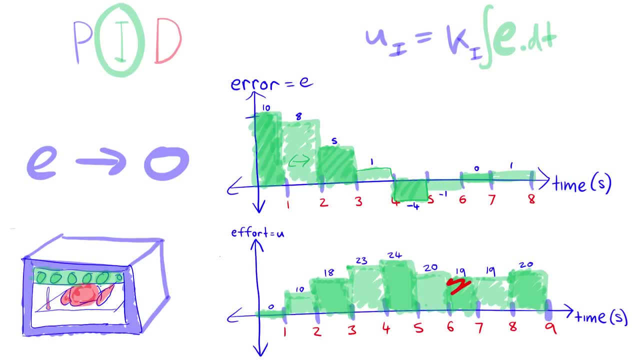 error reducing a little bit. That again lowers our control effort to 19.. And after the next sample we've finally got zero error. but that's not the end of the story, because our control effort is still greater than zero. So effort does converge to a value above zero. It needs to keep heating. 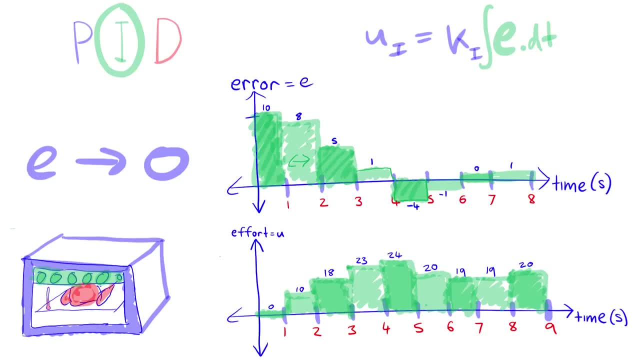 but it should be stable at some point, and it isn't yet. At the next sample we notice it's gone up to 1, and that area adds to 20, and at that point the oven's temperature is stable. Apparently, it's the fastest heating oven in the world: It's heated up in 8 seconds. 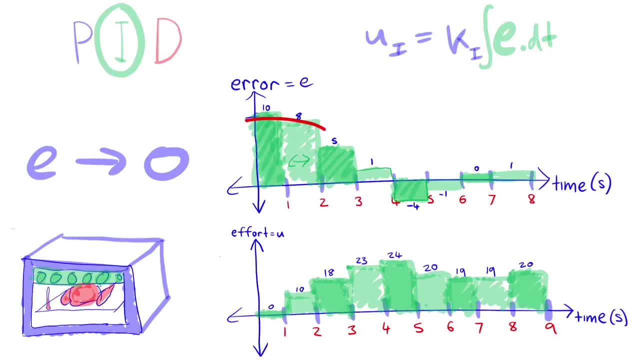 so really great. Notice that the waveform here ends up going like this a little bit and that trough there here is called overshoot, And this is something very um, this is a problem that integral controllers face. They have a thing called integral windup and this is the building. 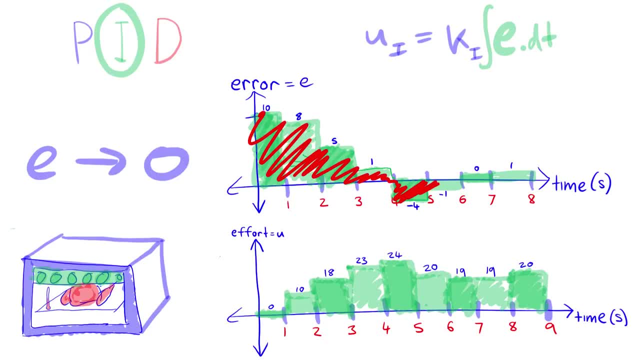 up of this area here behind the current reading. And there are lots of ways to deal with this. Um, many controllers just say you will never have more integral windup than value x. So if your limit was x, it will just limit the the possible um integral value. So if your 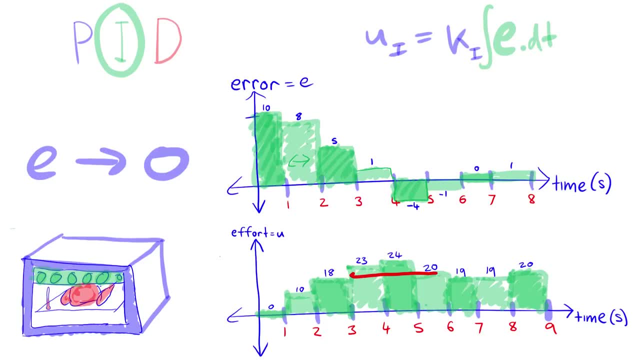 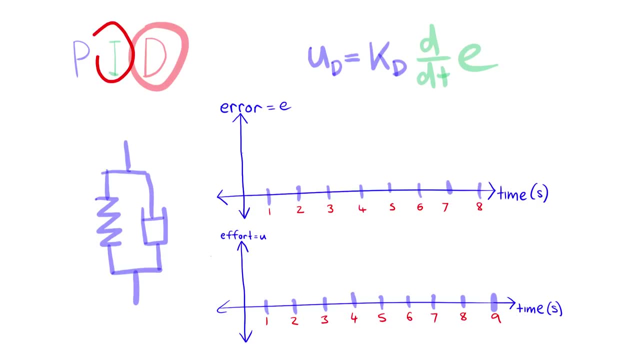 limit was was 20, um, then this would just limit it to this Um and it would never go above 20.. We've talked about proportional controllers and integral controllers, and from proportional controllers we get our response speed- how fast the system will respond- And from integral, 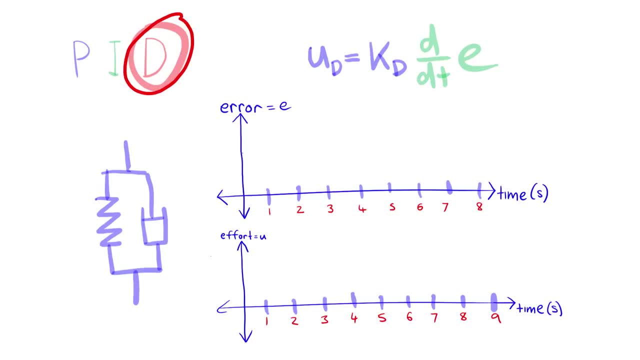 controllers. hopefully we get zero error, So why would we want a derivative control? It sounds like we've got what we want. Well, not quite In the scenario where you've got a steady state system, it's reached steady state and we've got this nice solid line. you want to be able to reject disturbances. 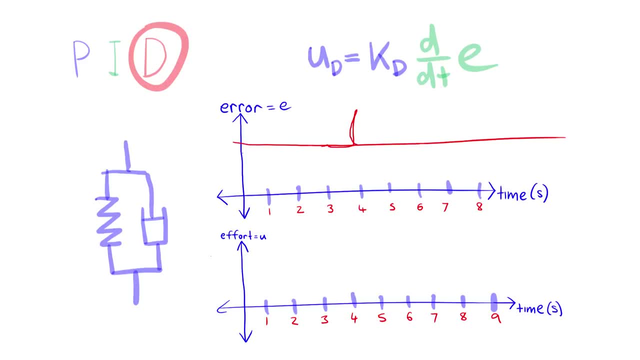 And what is a disturbance? Well say, someone sneezes in front of a pendulum and then the error goes like this: With an integral controller, it takes a while for the system to build up any control effort, So the integral controller doesn't really respond well in this situation. 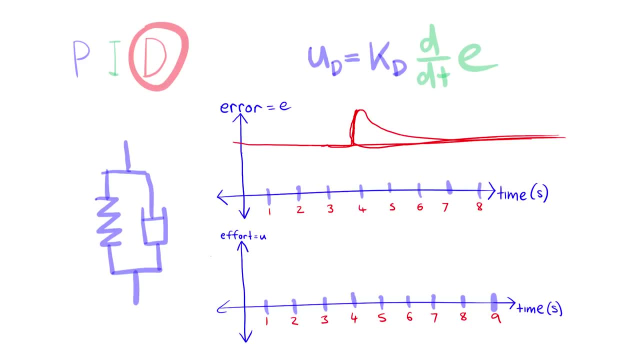 In this scenario at all. With a proportional controller it does respond, but proportional controllers don't- um, they don't have the response speed before the the value ends up getting large. A proportional controller is just the constant times the error. 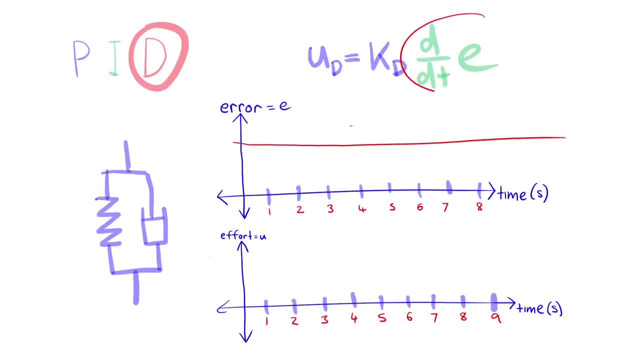 So what do we do? Well, what we can do is take the derivative, That means the rate of change. And what is the rate of change when the someone sneezes in front of a pendulum? It's very high. So a very high rate of change. we get this nice. 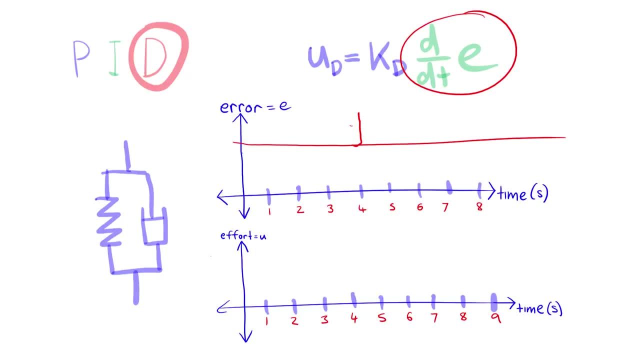 opposing. well, it could be. depending on the sign of the constant, we get this nice opposing force that as soon as a disturbance occurs we can resist it and move back to our set point and allow the integral controller to resume its normal business. Now there are problems with derivative controllers, really big problems, And these are mainly 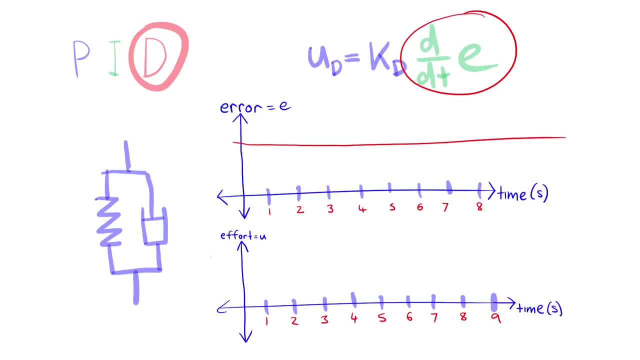 the limitations of sensors, the digit discretization and all kinds of things like that mean that the system is very noisy. So what we can do is we can put in a control effort from the line you end up taking the rate of change of noise, which ends up being well pretty damn noisy. So you keep putting. 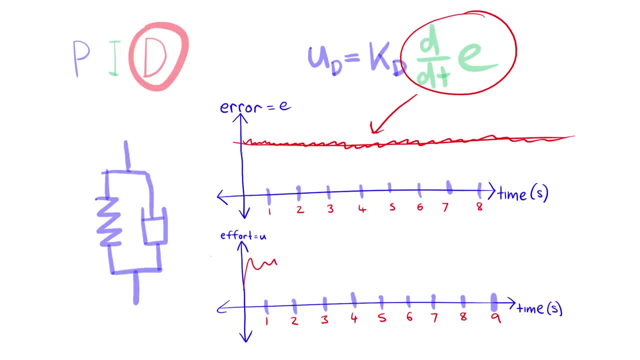 control effort in um which which is from the noise, and you don't really want to be doing um this, this sort of thing, because it ends up causing kind of like a instability in the system. It makes the system very noisy and audibly noisy in the case of pendulums. 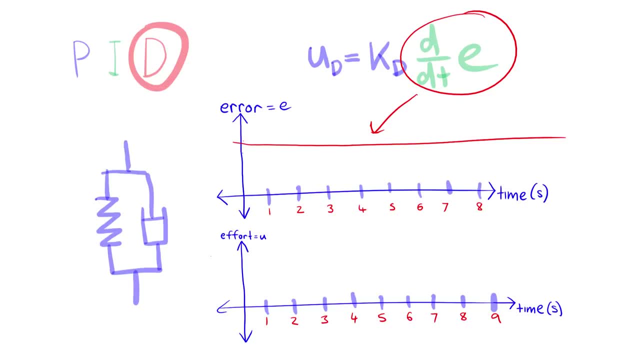 and in the case of cruise control, the vehicle would be like shaking or something. An example of this equation is actually in the damper. A damper is something that absorbs energy and it stops um endless oscillations and things, And this is actually the same form. 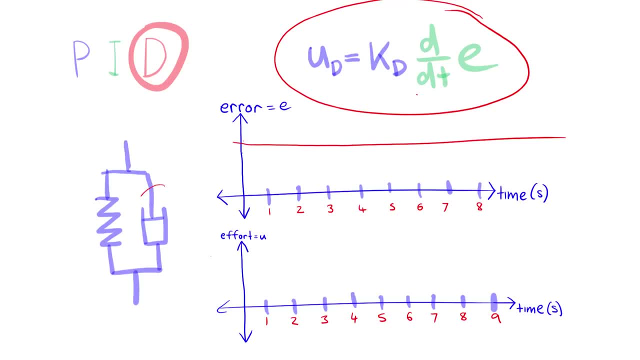 Um, the equation is in the same form as the damper equation. That's the equation that represents this mechanical element, And these are. this is a uh fundamental element in car suspension. If you just had a spring, you'd be bouncing all over the place. If you 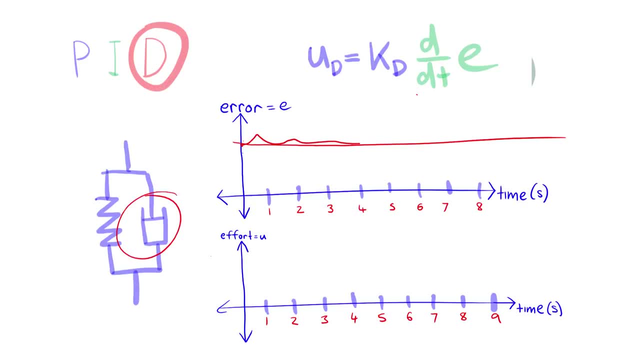 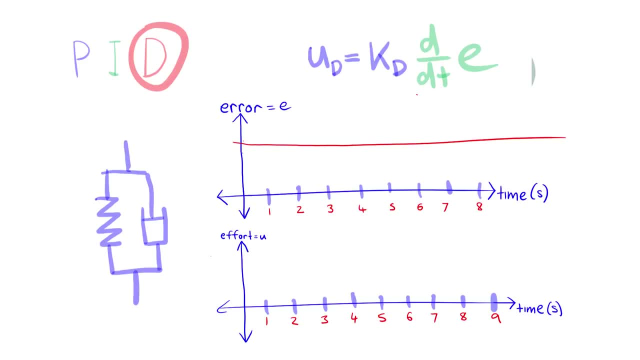 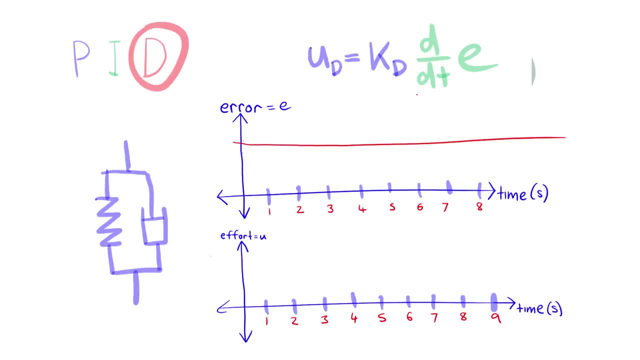 That is, that can be a pitfall. The derivative component can also help to reduce the settling time of a system. Um, this is improving the settling time component. it acts against change of error. So if the system has reached its set point. 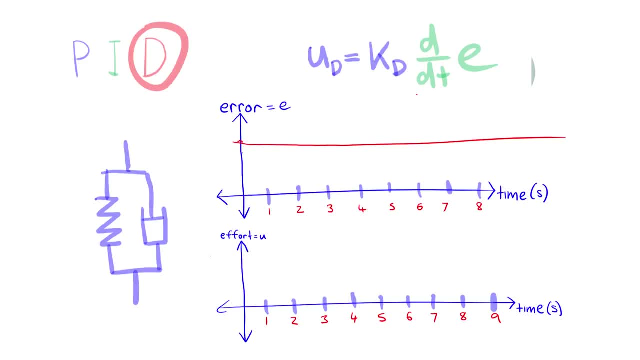 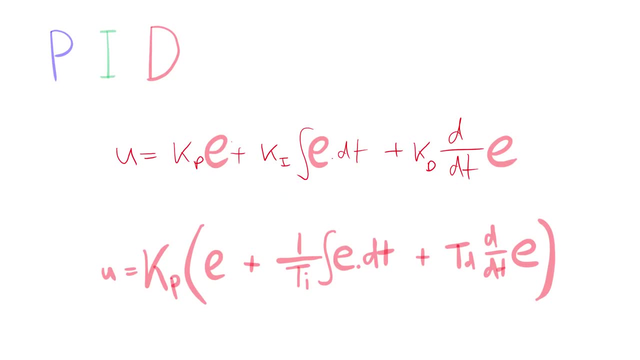 then it's going to resist any change away from that set point, and this includes overshoot. So this is the equation, which might be scary to some many. that represents a PID controller, The proportional controller added to the integral controller, added to the derivative controller. 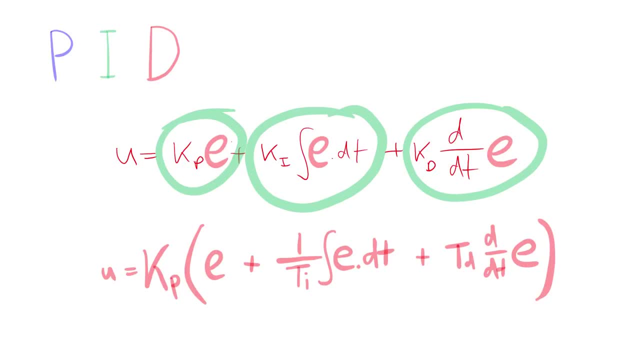 And now this form isn't what you see in control textbooks very often, because the form here is actually easier to work with with a process called tuning. Tuning is the process of improving the constants in front of the controllers: the proportional, integral and derivative. 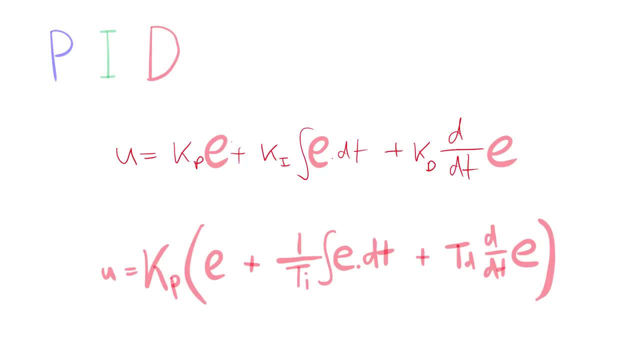 controllers to improve the response of the system. You might want it to respond faster to disturbances, You might want it to reach steady state faster, You might want it to be slower, And this form makes tuning a bit easier because it allows you to use a process. 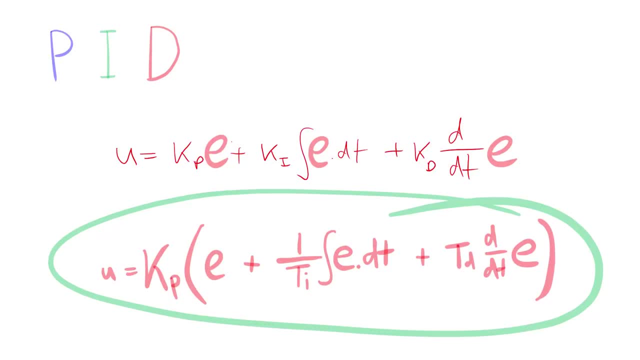 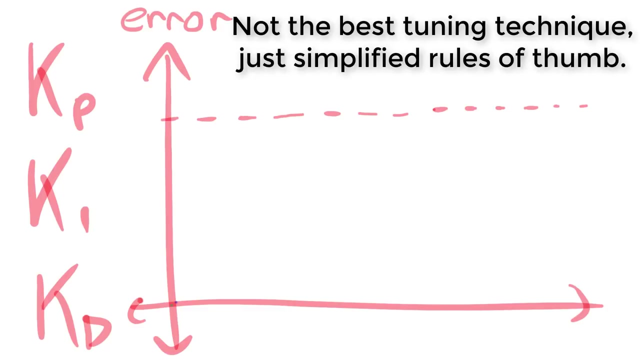 called Zeigler-Nichols tuning, which gives you a starting point for the values of these constants. You wouldn't want to rely on just that process, but it does give you a starting point for the constants in front of the components. So let's talk about tuning. So if we have a response that looks like this, what should? 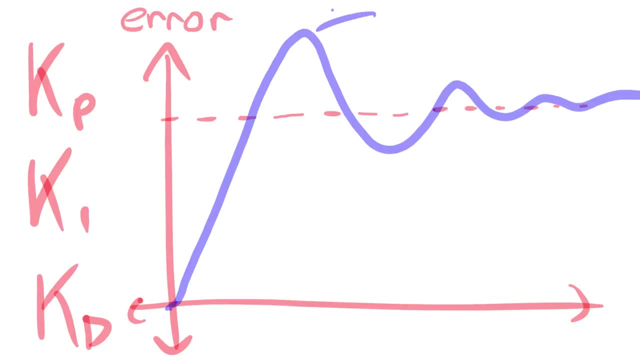 we do Well in this scenario. we don't want it to ring like this. We don't want it to have this period here t d. We don't want it to have that. We want it to look like this: 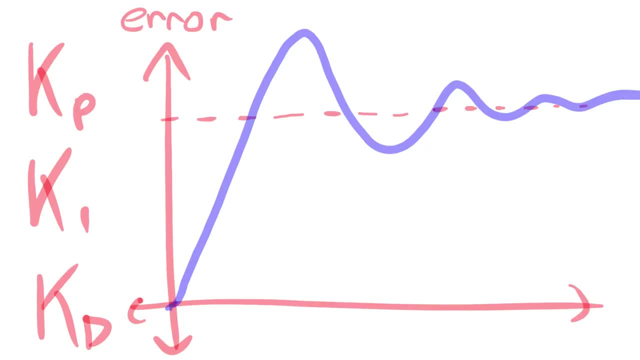 We've got our constants from the Zeigler-Nichols tuning process and we want to improve it. We want to make it closer to our shape. So what do we do? Well, oscillations like this are caused by the component of the integral and the proportional. 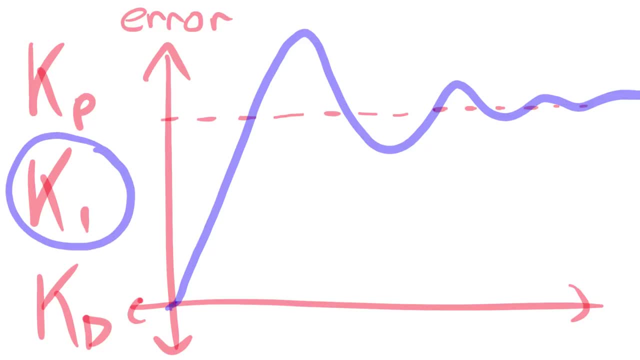 component. And if the integral component is a dominant component, then it's very likely that integral windup is causing this overshoot. So let's try to reduce our integral component Now. it's likely that you end up with something like this, And that might not still be with your response. so you notice that the integral component 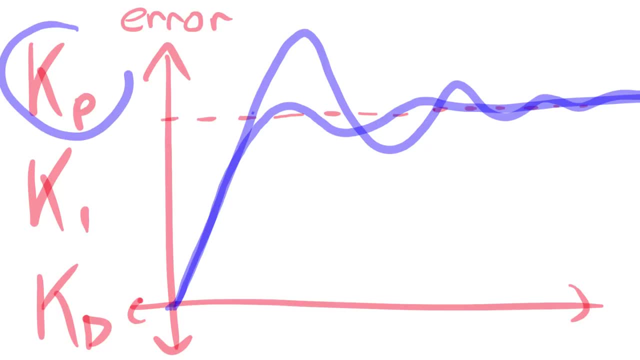 is no longer significant, And that's because the integral component is a dominant component. So now let's reduce the proportional component. Now that doesn't oscillate anymore, but we do want it to perform a little bit faster. So what do we do? 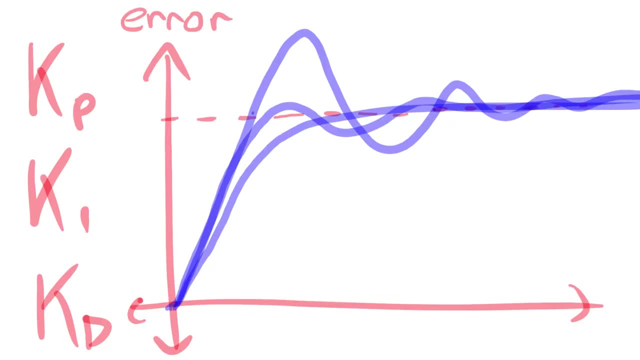 Well, the integral component. now we can change it and probably we can increase it. We know that our value of the integral component is somewhere between the constant that it was initially and after our tuning. So let's take the average of those two values. 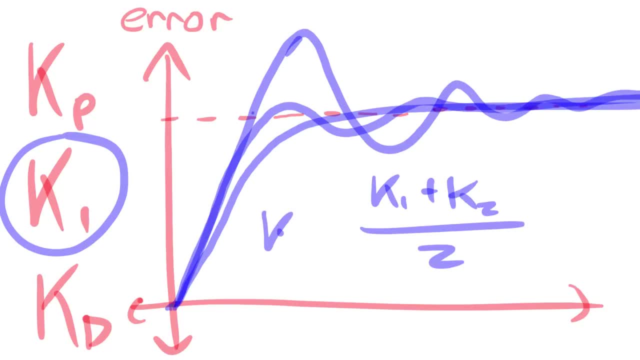 Let's call them k1 plus k2.. And we're going to reduce the integral component, We're going to reduce the integral component And we're going to reduce the integral component And we're going to reduce the integral component, And that will be the new integral constant. 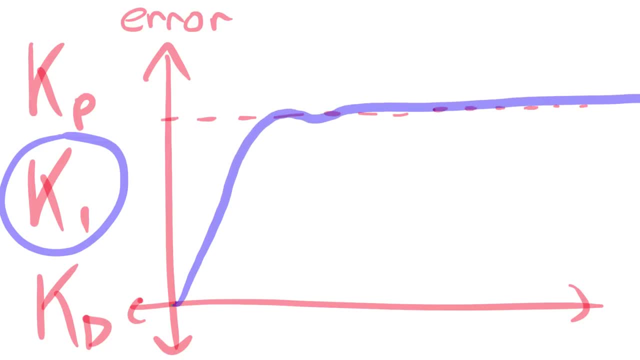 And now we probably will get a little bit of overshoot. But now we've got that response time, Now we haven't really got any derivative component yet. So we now want to start working on that. We're now testing our disturbance rejection. 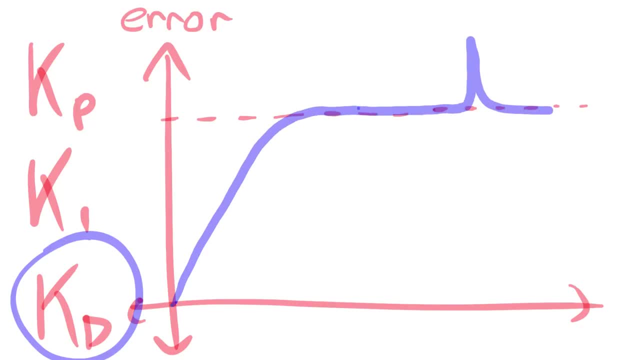 So now we're testing the response to disturbances. So we start bumping it And we notice that in the normal case it decays really slowly. We want it to behave like that first curve, So we increase the derivative component so that it's still relatively insignificant in. 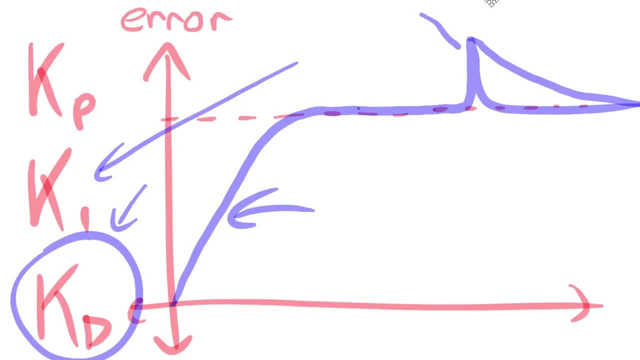 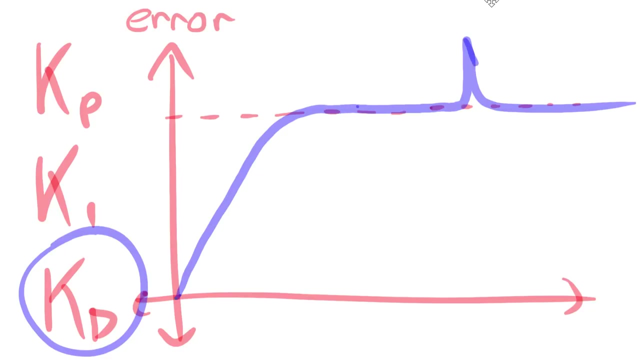 the initial curve. But when there's huge rates of change like this, it has significance. It is more significant than a proportional component. So we increase the value, maybe by a few percent, 10% or something, And then we see how that response ends up. 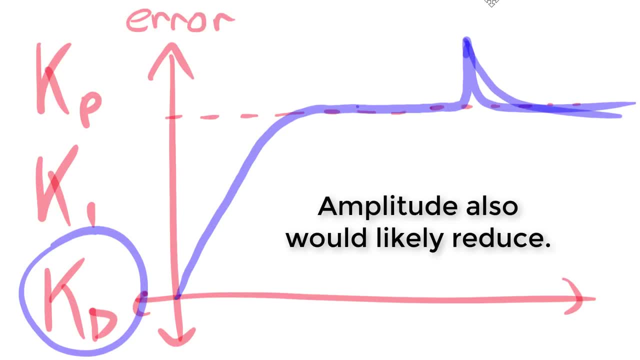 And you'd probably end up with something like that. So you do it again And now you notice that you end up with the response you want As you slowly, iteratively, improve the coefficients. Now, each time you change one of these variables, the response you're probably kind of wrecking. 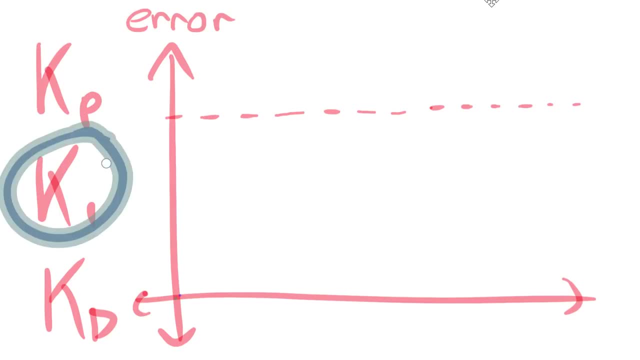 your tuning for the other variables, So you have to retune those as well, And this process is an iterative process. You slowly improve it And there's actually an absolute ton of methods of doing this. There's probably thousands of them. There are tons of methods to get the initial values. 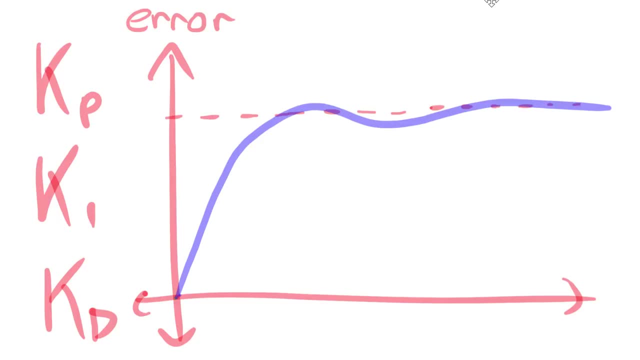 And I think Zeigl and Nichols. the ultimate cycle method is probably the easiest And I'm going to show you how to use that in a moment. We know how to tune, but we don't know how to get a starting point. 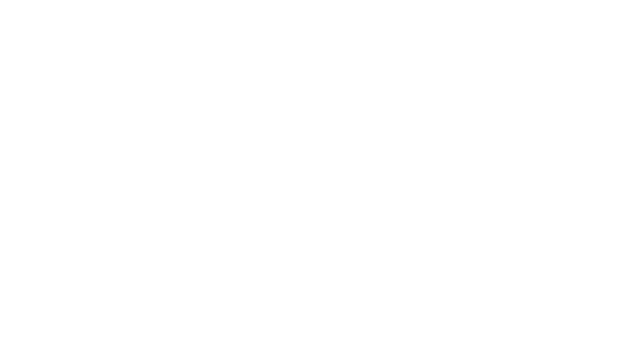 What are we tuning from? Well, the way to get a starting point is to do the following. In most systems- well many systems- it's acceptable to test the unit a fair bit before you end up having to use it. So what we do in this process is we have the unit with just a proportional controller. 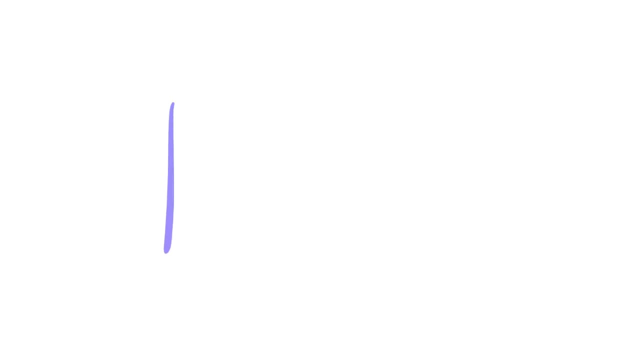 We have, let's say, the oven, And we have the oven with just that proportional controller. So we have this oven And we've got that digital controller sensing the temperature and adjusting the oven accordingly. So what do we want to do? 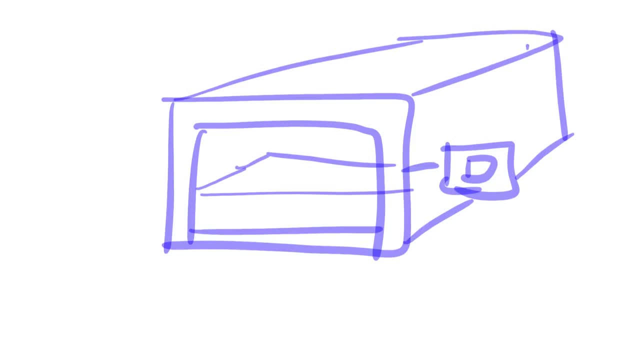 Well, if we make the proportional component too large, then we end up with a system that does this And the response gets these ever-increasing sinusodes, And this is very unstable. This is the basic definition. This is the definition of an unstable system. 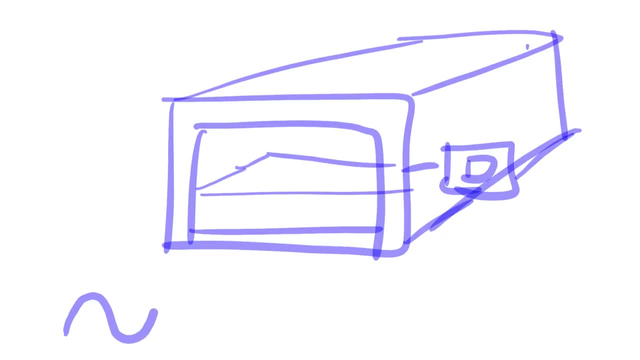 What we want to do is have it a stable sine wave, so that the amplitude is roughly not changing. Actually, that's the way normal Zeigler-Nichols has done, but I think you should probably aim for something that is stable but decays extremely slowly. 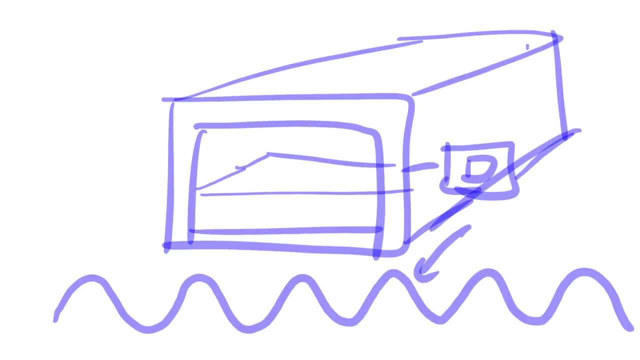 You're looking at the error and you want the error to have this just constant sinusode, which might seem a bit weird because that's exactly not what we want to happen. but this is how we do this. We start off with a constant for Kp, the proportional controller, that just oscillates. 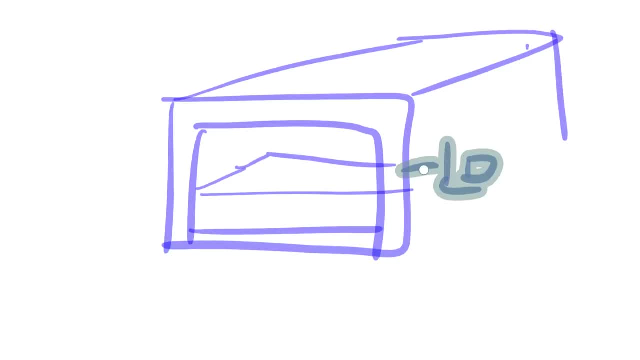 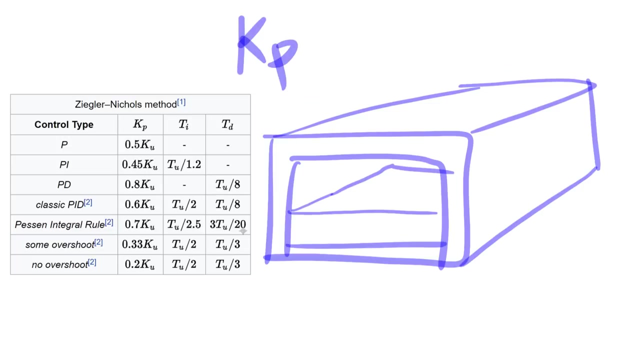 like this. Now, when you have this constant, you can use the equations that many have come up with that use this value to create a starting point for your system's controller. From before, we have our Kp value, And when the Kp is equal to the gain that results in a sinusode, it's greater than the. 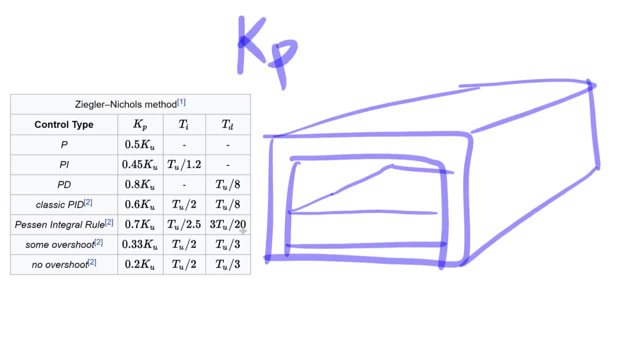 value of the Kp stable sinusoid. then it is called Ku, So Ku is the gain at which you've got a stable sinusoid. Now, presumably you can measure the sinusoid's period. I assume you can measure the sinusoid's period and that value is quite important because we're going to use it in. 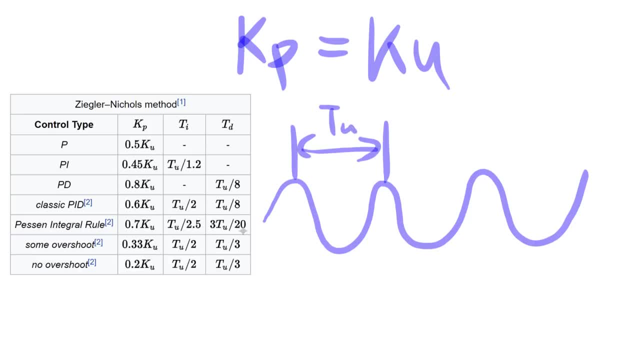 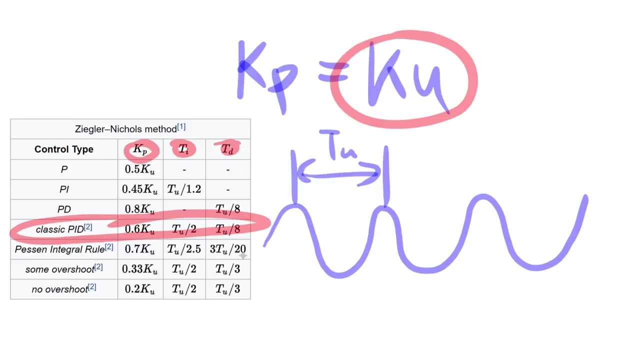 this tuning method and that value is called Tu. With Ku and Tu, you can use them in this equation here to get default values for the controller coefficients. So 0.6 times the value of Ku is the coefficient for the proportional controller and you can use that value as: 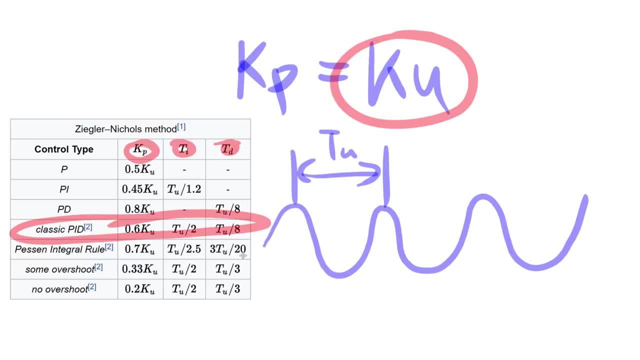 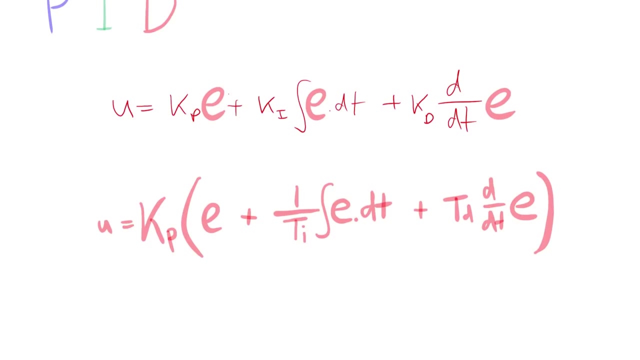 a starting point: Tu divided by 2,, that's the period divided by 2, is the coefficient for the constant for the integral controller, and the period divided by 8 is the coefficient for the constant in front of the derivative controller. So that actually gives us everything. 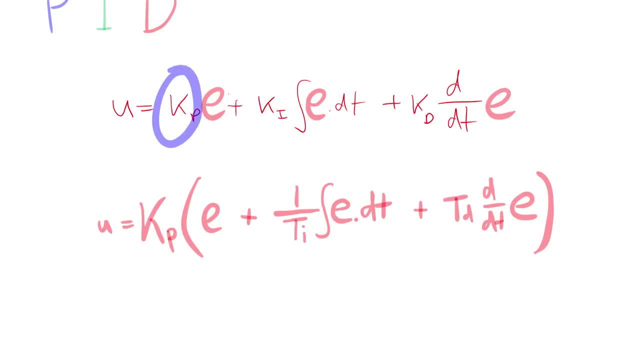 We now have an initial value for Kp, Ki and Kd, because we have an initial value for Kp, Ti and Td, And to tune the values all you do is expand this equation and then you can tune the values in front of the controller, as if you had the controller before, And it's 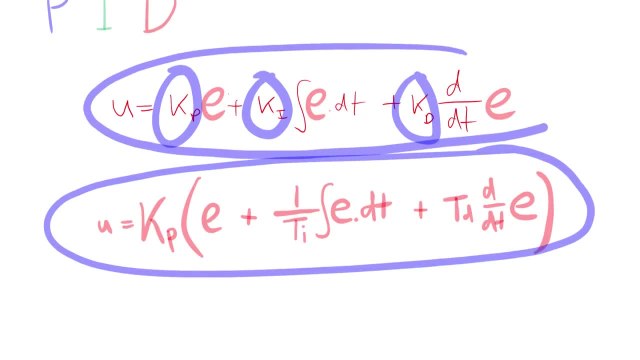 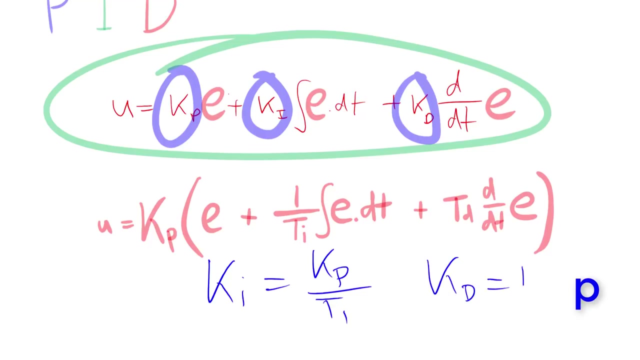 much easier to do The iterative improvement tuning on this equation than it is on this equation, in my opinion. So after you get these Ti values and Td values, I would convert it to the form you see above here. That is simply by doing this You just do: Ki equals Kp on Ti and Kd equals Td, Kd. 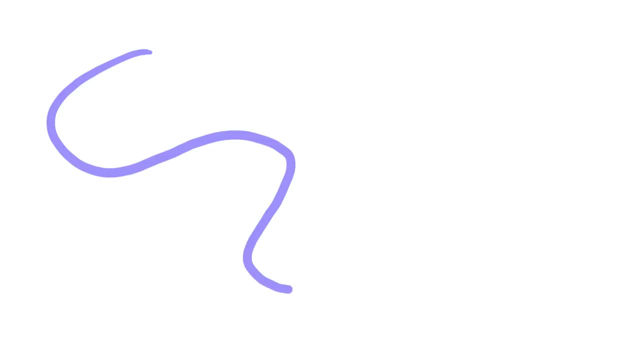 And that's it Now. I am aware that the control theory can be a little bit dry, So this is just the start. This is the boring part of this. What we have coming is a nice little inverted pendulum balancing robot which will just wander around the office balancing, And this is going to be designed 3D printed. 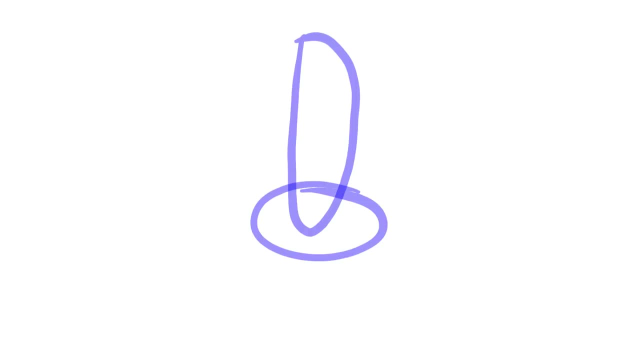 and then we're going to use that Zeiger-Nicholas tuning to just get it to balance in an empirical way. If anyone wants to know more about this, leave them in the comments below And I'll see you next time. If anyone wants to know the theory, the mathematical, the theory behind this and how you can derive,